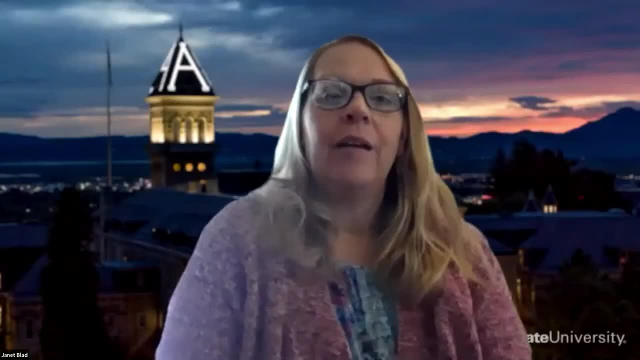 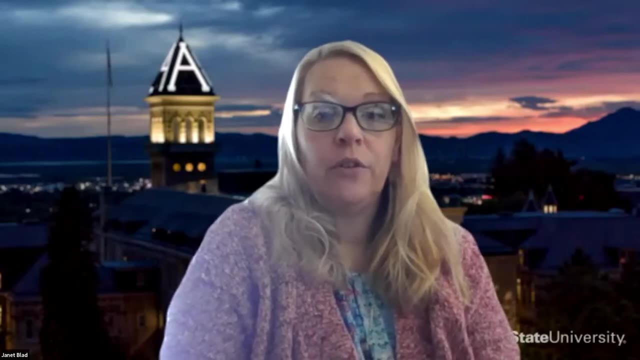 Hi, my name is Janet Blood and I am with Utah State and I'm in the Biological Engineering Department and I'm here to talk to you for a few minutes about what biological engineering is and the opportunities you'll have at Utah State to participate. 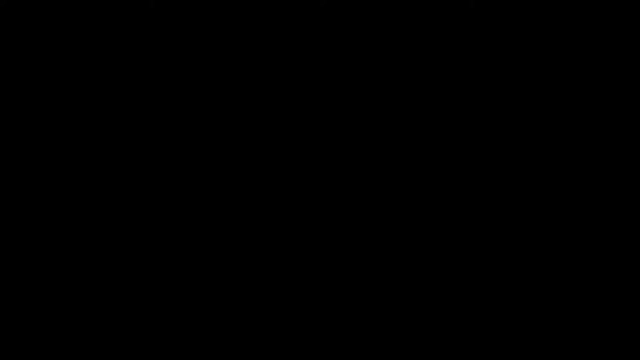 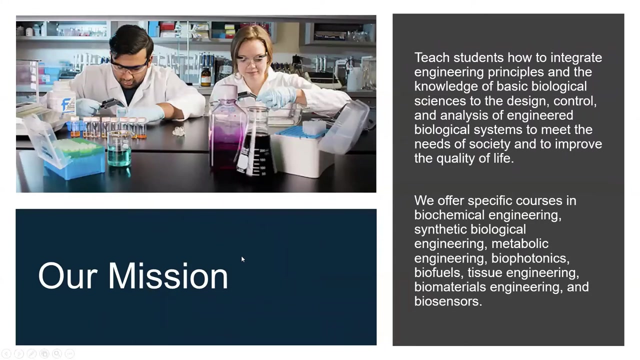 I am going to share my screen with some slides about biological engineering at Utah State. Our mission is to teach our students how to integrate engineering principles and the knowledge of basic biological sciences to design, control and analysis of engineered biological systems to meet the needs of society and to improve the quality of life. 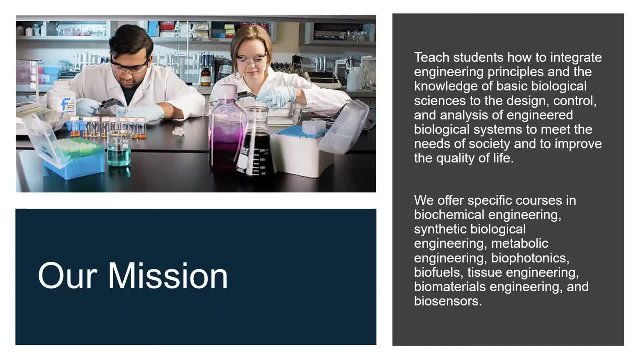 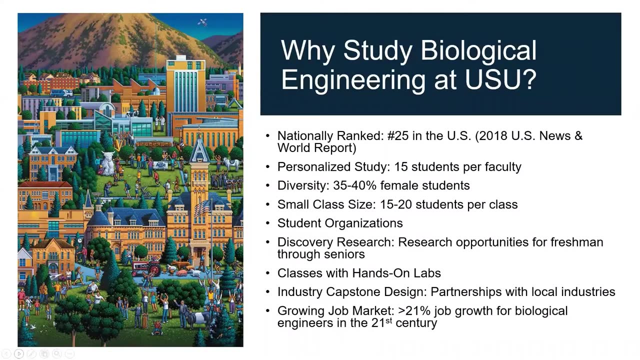 We offer courses in biochemical engineering, synthetic biological engineering, metabolic engineering, biophotonics, biofuels, tissue engineering, biomechanics, and material engineering and biosensors. Why study biological engineering at Utah State? Well, number one, we're ranked in the nation. 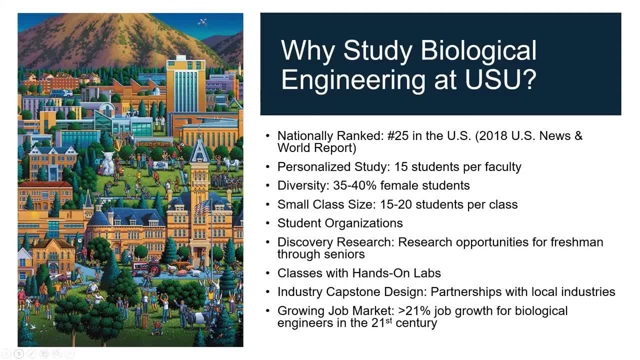 We have personalized study with about 15 students per faculty. We have a pretty diverse population, with about 40% female. We have small class sizes. We have fabulous student organizations. You have opportunities for discovery research from the time you're a freshman through your senior year. 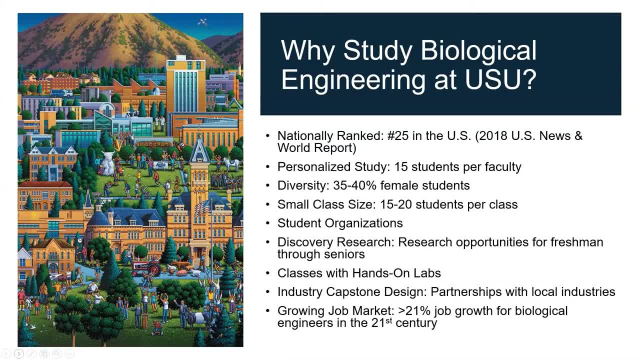 We have classes with hands-on labs. You go to your lecture, you hear and learn, and then you get to go to the lab and work on the activity. We have partnerships with our industry here locally, So our industry- Capstone Design- our students have the opportunity to interact with those that could potentially be their future employers. 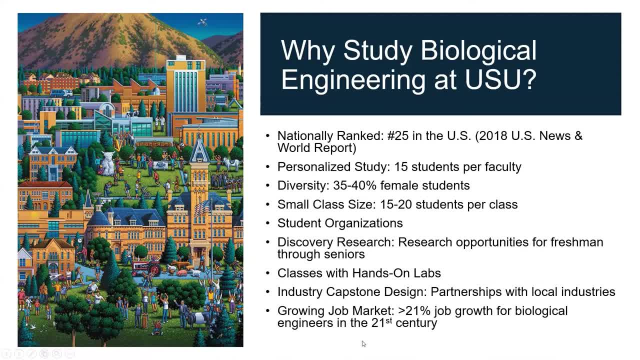 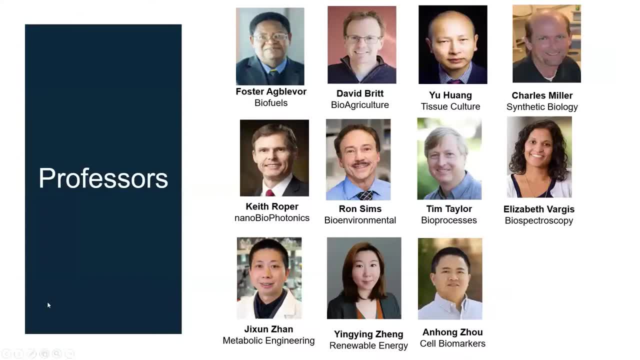 We have. there is a great growth market of free research. Our professors are the jobs in biological engineering. Our professors are very knowledgeable and enjoyable to be around. We have a great staff. Dr Aglabor is our specialist in biofuels. Dr Britt does bioagriculture. 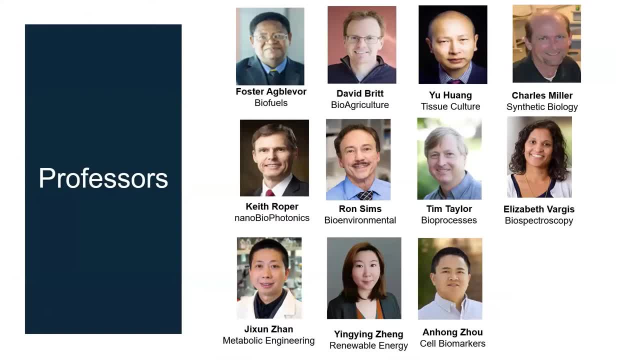 Dr Wan does tissue culture, Dr Miller does synthetic biology, Dr Roper does nanobiophotonics, Dr Sims does bioenvironmental, Dr Taylor does bioprocessing, Dr Varghese does biospectropathy. 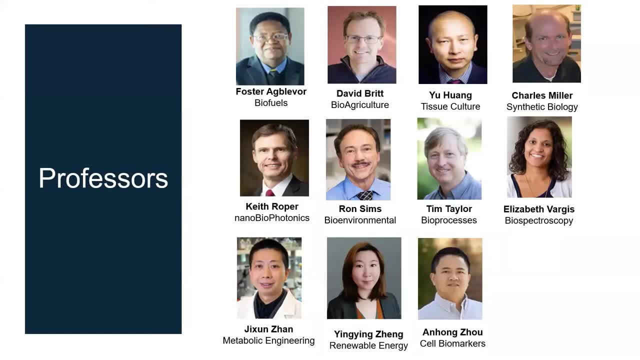 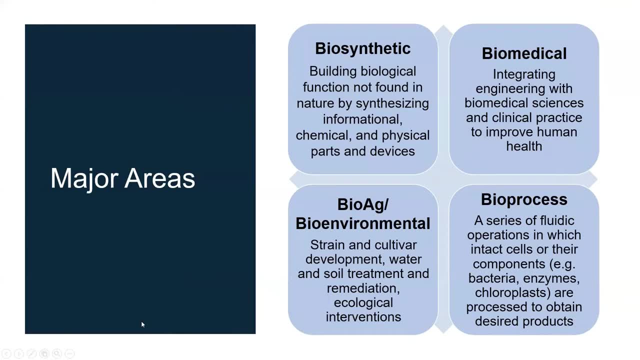 Dr Zahn does metabolic engineering, Dr Zhang does renewable energy And Dr Zhao does cell biomarkers. You have four major areas of study in biological engineering. Biosynthetics is building the biological functions not found in nature by synthesizing informational, chemical and physical parts and devices. 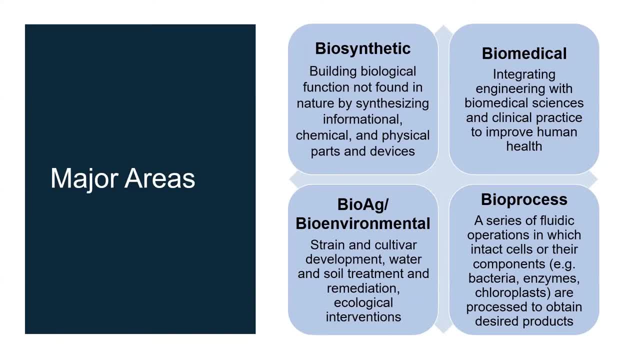 Biomedical: integrating engineering with biomedical sciences and clinical practices to improve human health. Bioag and bioenvironmental is strain and cultivar development, Water and soil treatments and remediation, and ecological interventions. Bioprocesses is a series of fluidic operations in which an intact cell or other components, such as bacteria, enzymes or chloroplasts, are processed to obtain desired products. 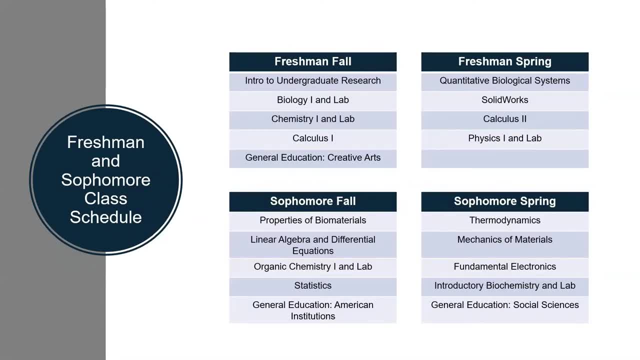 Here's a look at your classes for the four years that you're here at Utah State. You start out with intro into undergrad research, which is your BAME 1000 class, And then you get some chemistry and biology calculus in your spring. 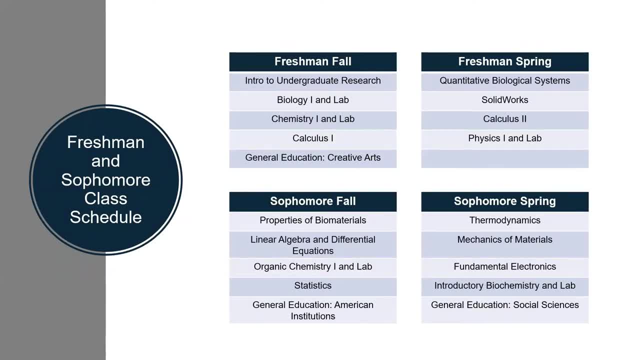 You get to do more biological engineering courses with solid works and quantitative biological systems, Some calculus and physics. When you're a sophomore you move into properties of biomaterials, which is your biological engineering course, And then several other courses. You get courses of algebra and chemistry. 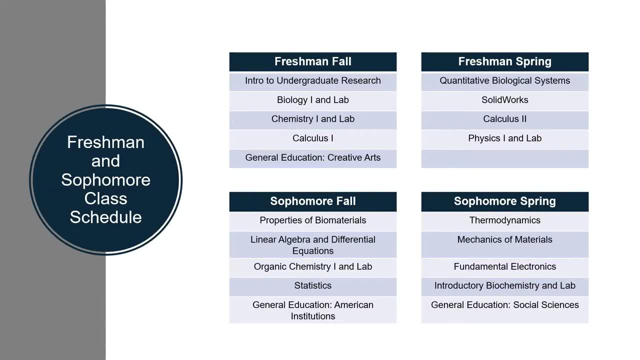 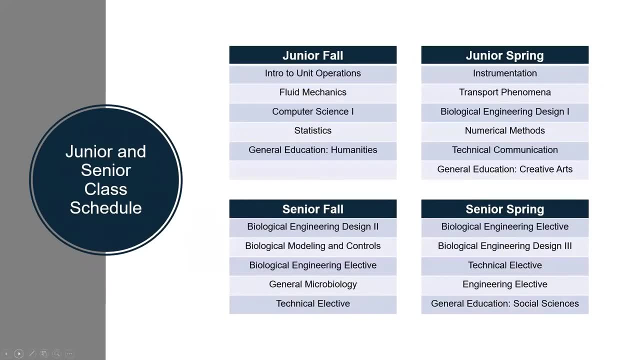 Your sophomore year. you get thermodynamics, that spring and mechanics and materials And get some other great courses Into your junior year: your intro to fluid ops, Your intro into unit ops And then you get your fluid mechanics. I always get those two names stuck in there. 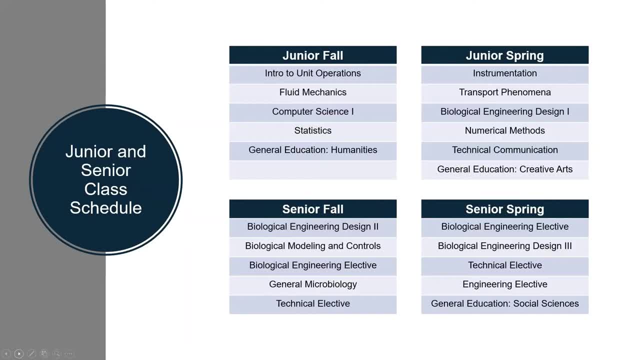 You have computer science and statistics. The spring of your junior year you start your biological engineering design one course which is your capstone project that you're working with a team for the next three semesters to come out with a project that is completed that you will feature at your senior design night. 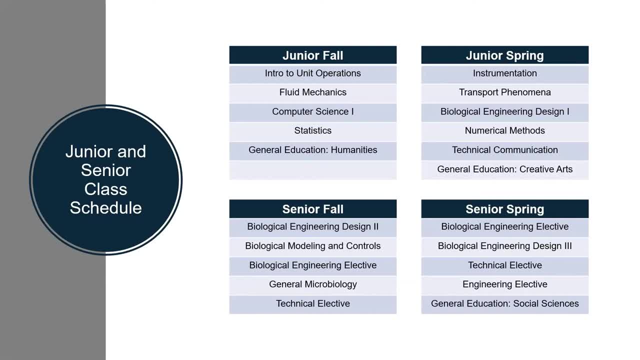 We have our senior. your fall in your senior semester You continue with your senior design And you get to take some electives And your spring you finish your senior design course And then you get your different electives that will finish out your degree. 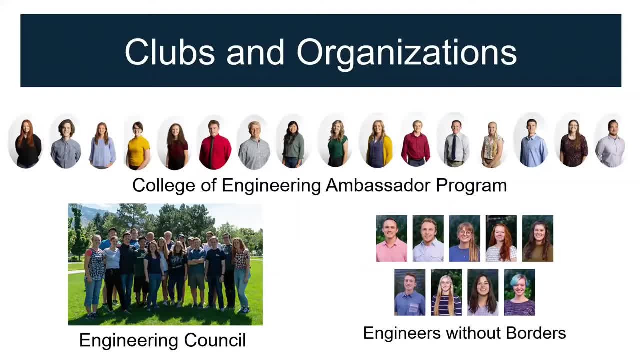 We have lots of opportunities for great clubs and organizations. on the college level You have opportunity to apply for an ambassador program And you're an ambassador. you get to mentor and teach other students. You get to go to elementary schools around and explain what cool things engineers do and help facilitate more information in students. 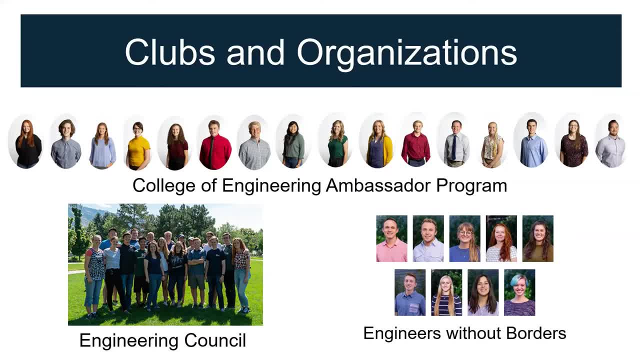 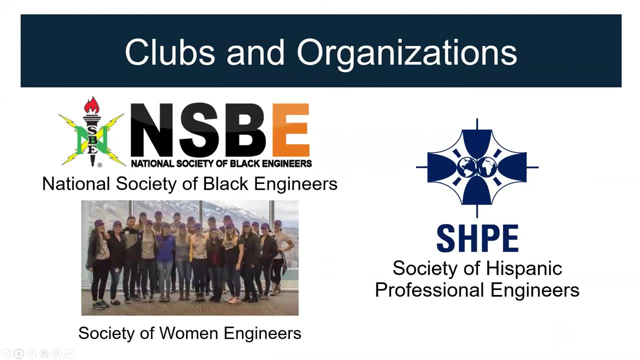 There's engineering councils so you get opportunity for service and leadership positions. Engineers Without Borders- another service opportunity, And this gets you around the world. We also have opportunities to participate in the National Society of Black Engineers, the Society of Women Engineers. 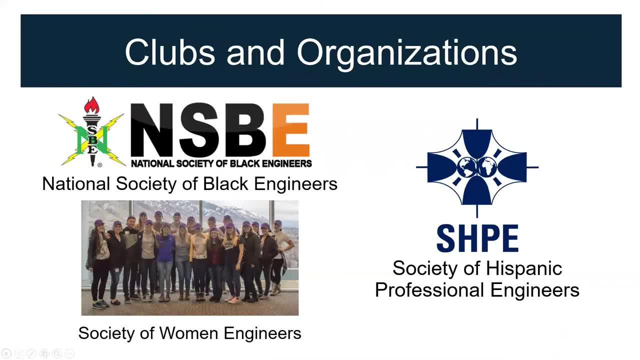 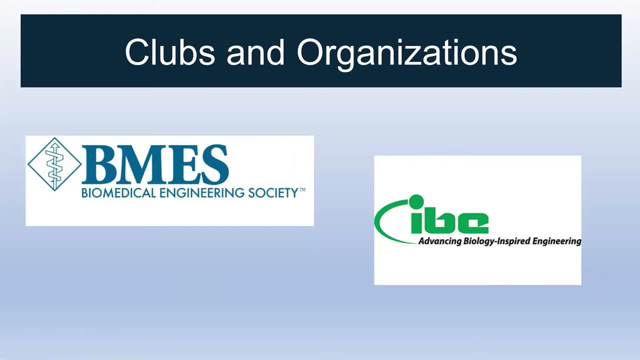 and the Society of Hispanic Professional Engineers. Those are all on the college level. In the department we have our own groups of Biomedical Engineers Society and the IBE, which is Institute of Biological Engineers. They have a lot of conferences and opportunities for you to go present your research, learn from others. 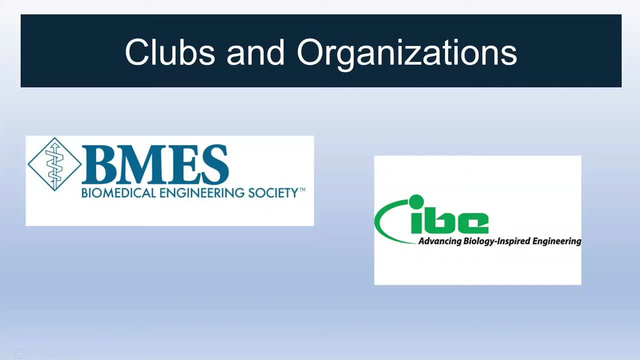 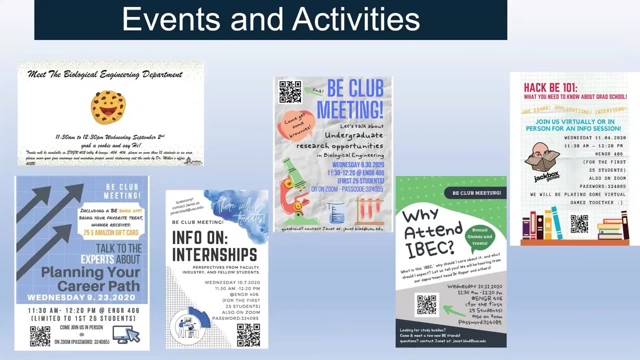 interact and get a really well-rounded resume and your college career. We had a few fun events this past fall that I wanted to highlight. We started out with a meet and greet- get a cookie. meet your staff, meet your faculty, meet new staff- interact. 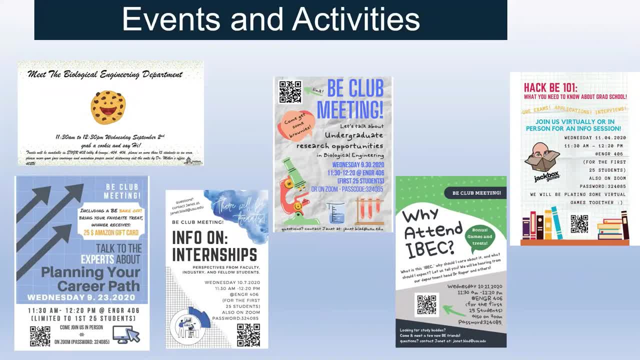 We had some seminars. We talked about planning your career path. We talked about internships, undergrad research opportunities. We had a meeting about our Intermountain Biological Engineering Conference that we hold each fall. It gives students an opportunity to again present their research, and why is it important to go to those type of conferences? 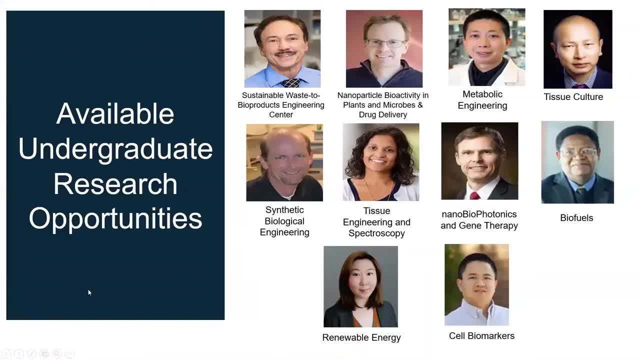 And then we talked about grad school. You have undergrad research opportunities. The department has lots of lab meetings weekly that you can attend and learn about what they're doing in their labs and then get busy and participate and do some undergrad research. Here's a career path. 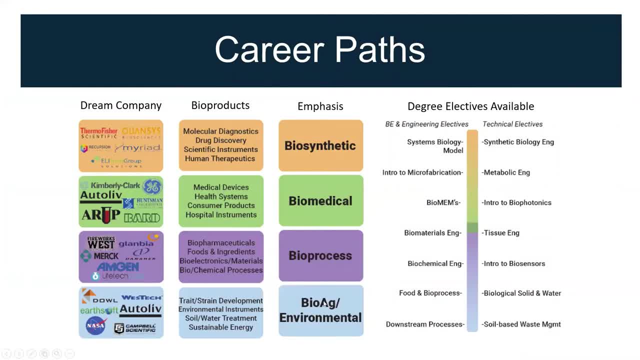 So, as I told you earlier, there's the four emphasis of biosynthetics and biomedical and bioprocessing and bioag and environmental. So those are different products that you get to do and work with And those are companies in the local area Intermountain West that you can work for eventually. 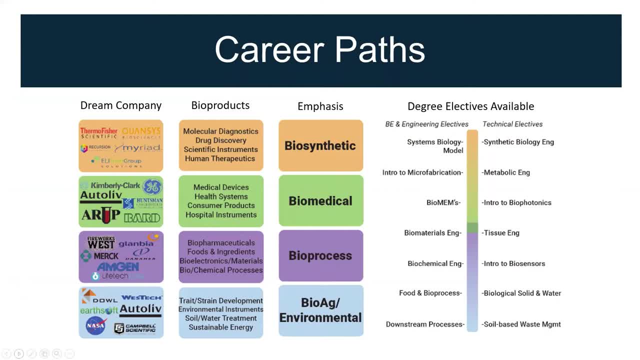 but you can find companies around the country, even around the world, that you could use your skills for. I talked about electives, So if you're more interested in biomedical things, then you're going to want to take Biomems as an elective in your upper classes. 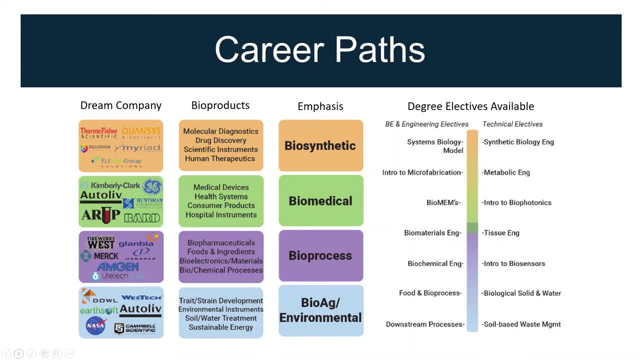 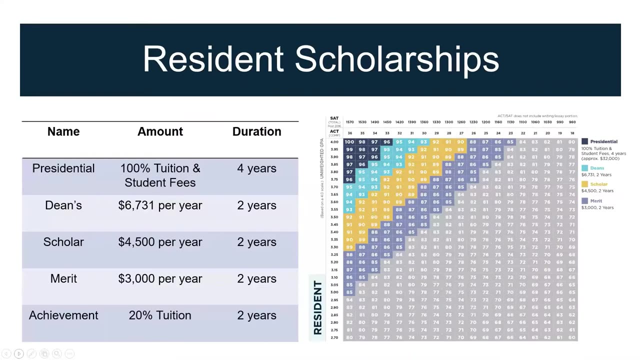 If you are interested in bioprocessing and foods, we have actually a bioprocessing foods class- Super interesting. So these are opportunities, These are the electives that you're able to take and how they line up and help you. You want to know about scholarships. 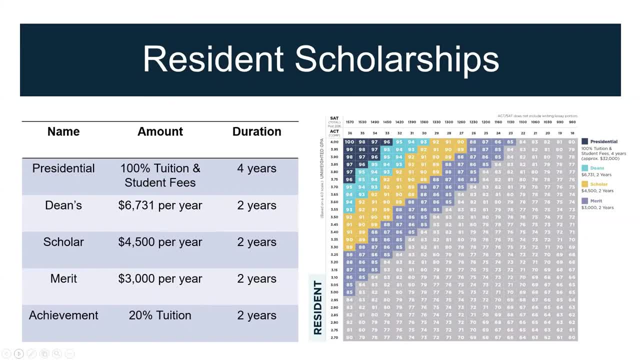 So resident scholarships- I've got both sides. I have a little graph of what your ATC's ACT score or SAT score needs to be, along with your GPA. I know currently the university is not requiring to take those tests to enter the university for fall. 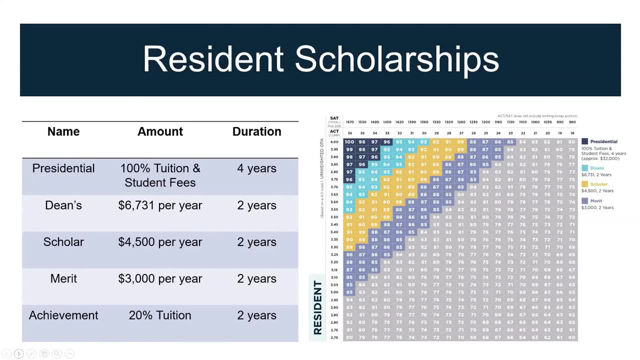 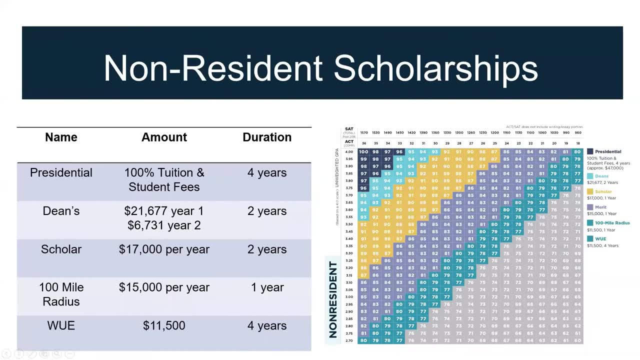 But if you want scholarships you're going to have to take the ACT or the SAT. So if you get, you know, the presidential scholarship, that's four years of paid tuition. Next screen: Oh whoops, The non-residents. again same thing. 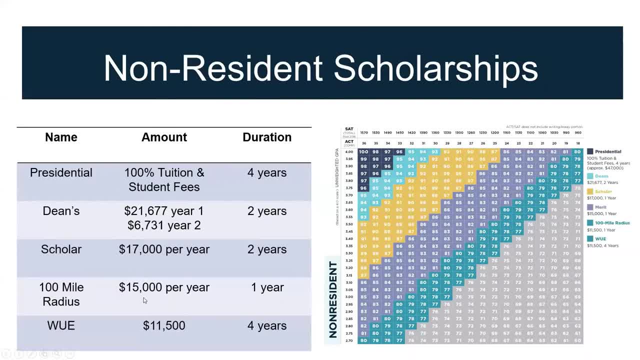 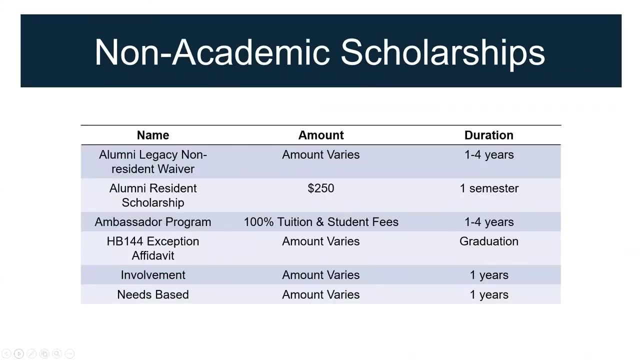 Here's how those all line up with what they offer. They do have this WUI scholarship, So if you're in the western states, you can still get access to reduced tuition. Non-epidemic scholarships are also available. One of the big ones is the Legacy Scholarship. 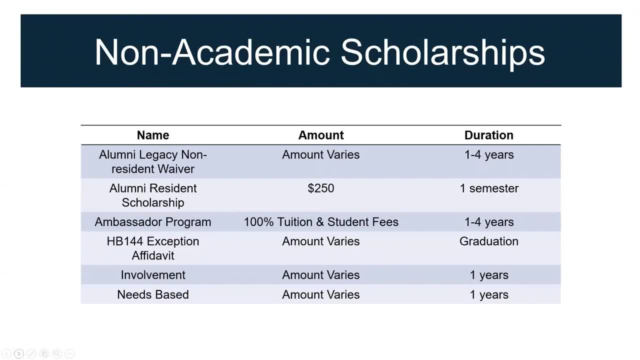 Which, if you're at a school, if you're in a state, it gives you in-state tuition And in-state you get a lump sum one time for tuition And the Legacy is that you have had a parent or grandparent attending the university. 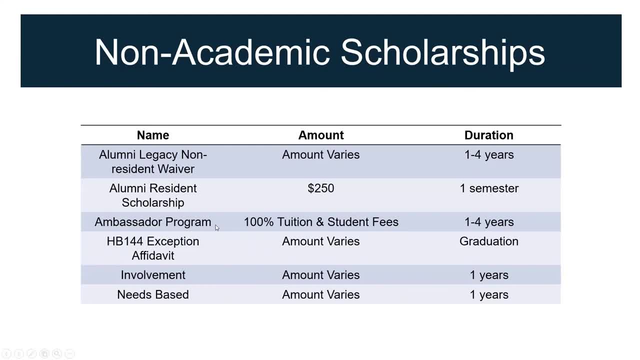 And then there's other programs that you can: This ambassador program. this is a university ambassador, not the College of Engineering. You do get a paid position for the College of Engineering. The ambassador program through the university is actually a scholarship that will pay your tuition and fees. 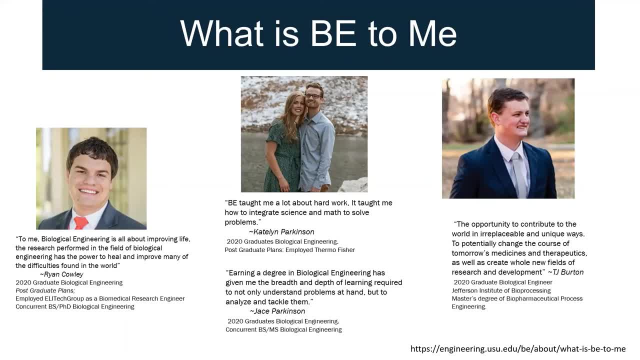 What is BE to me. So what is biological engineering to me? This is a clip of some students that graduated this past spring And I've just chatted with them And here's their quotes. The first one here is Ryan Kelly And he says to me: biological engineering is all about improving life. 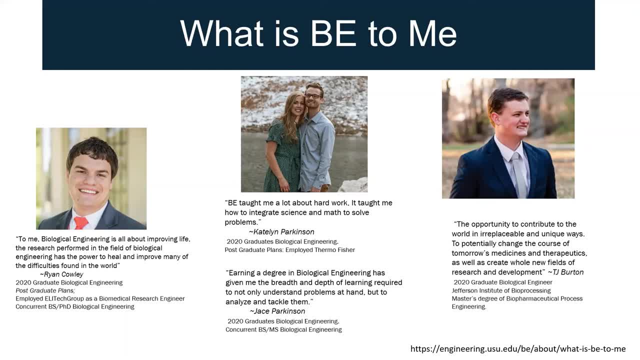 The research performed in the field of biological engineering has the power to heal and improve many of the difficulties found in the world. Ryan is currently employed at Eli Tech as a biomedical research engineer And he is participating in our BS and PhD program. 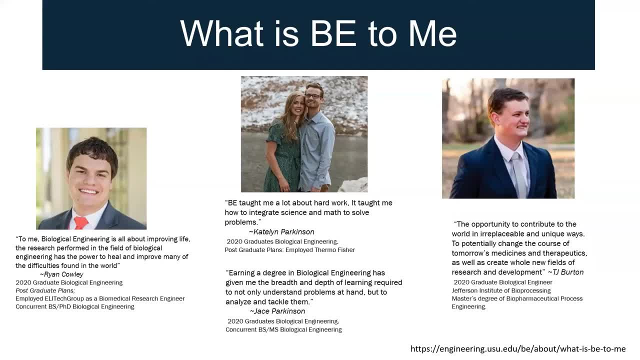 So he's working on his PhD. The concurrent program allows you to cut out some time and it's a little more of a fast track to continue. So he has his BS and he's working towards his PhD. This cute couple in the middle this is Jace and Caitlin Parkinson. 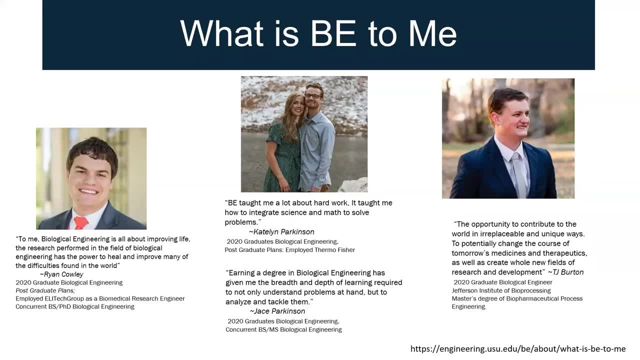 And yes, they met and fell in love while they were undergrads, So you can find your soulmate in biological engineering. Caitlin says: BE taught me a lot about hard work. It taught me how to integrate science and math to solve problems. 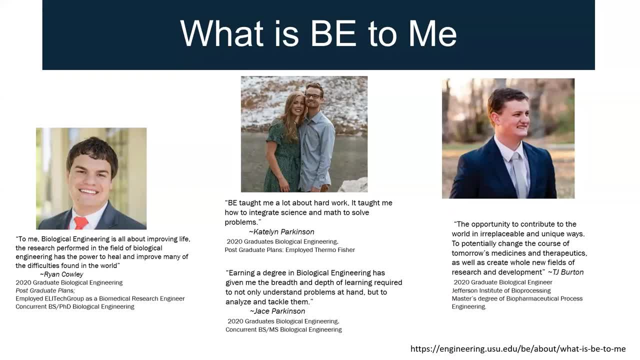 And she is currently employed at Hummel Fisher here in the Valley. Jace is participating in our BS and MS biological engineering, So he's working towards his master's degree and he is slated to be completed in the summer of 2021.. 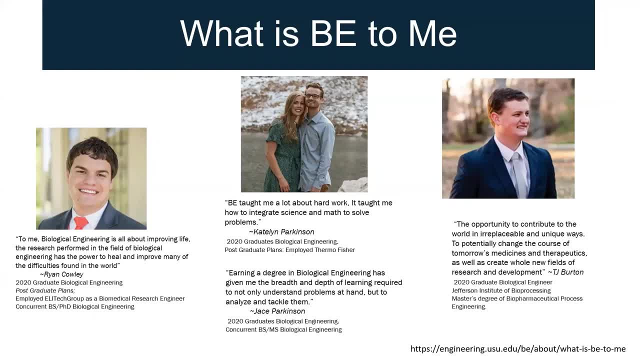 So this summer, And Jace says about biological engineering. Earning a degree in biological engineering has given me the breadth and depth of learning required to not only understand problems at hand but to analyze and tackle them. And our last student that I featured here this is TJ Burton, also a graduate from the spring class. 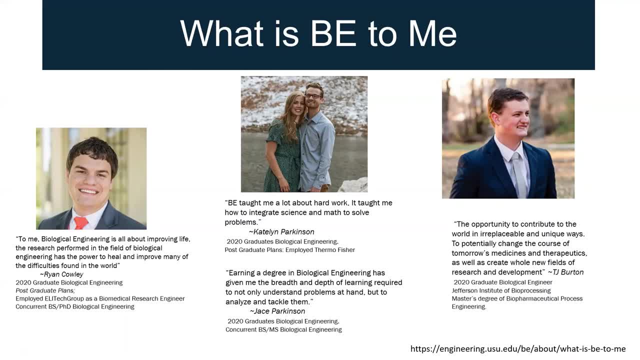 And TJ says, the opportunity to contribute to the world in irreplaceable and unique ways to potentially change the course of tomorrow's medicine and therapies, as well as create whole new fields of research and development. He is currently attending the Jefferson Institute of Bioprocessing.